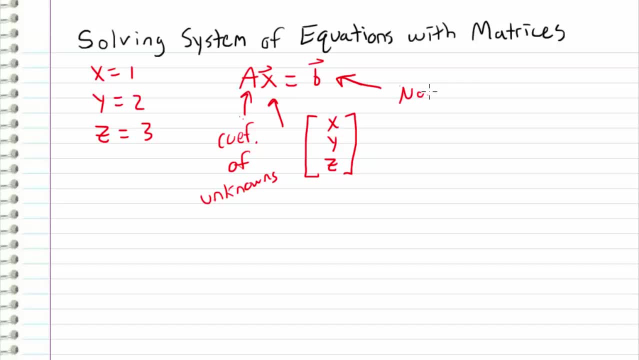 And that leaves this vector b as the non-coefficient numbers that are included in our three equations. But obviously this is a trivial example. Technically, we do have three equations. We have: x is equal to 1, y is equal to 2, and z is equal to 3.. So let's look at the. 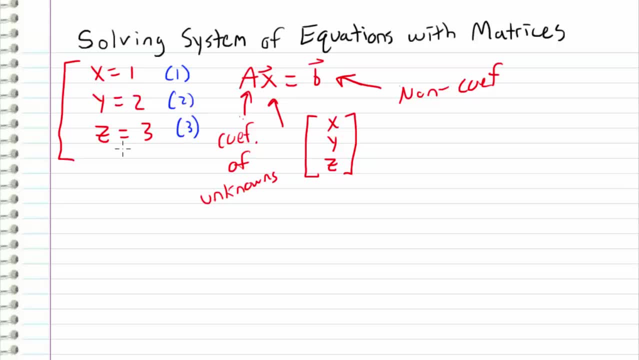 to 1, y is equal to 2 and Z is equal to 3. 1, 2, 3 equations. so if I wanted to organize this system into: ax is equal to B, well, I can do that, like this times: X, Y, Z, and this is going to equal the right-hand side of our equation: 1, 2 & 3. 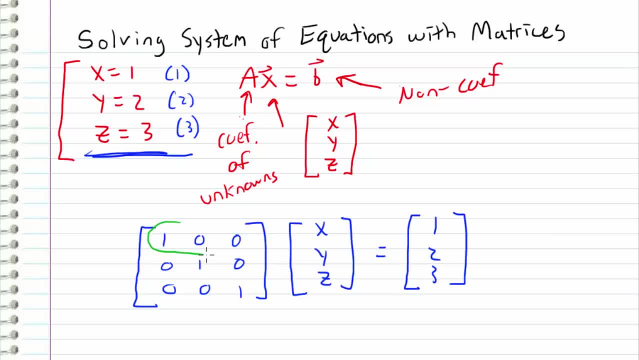 and let's verify that this is in fact true. if I were to take this first row and multiply it by our vector, what I would get is X. and if I were to take this second row and multiply it by our vector, what I would get is Y. and then if 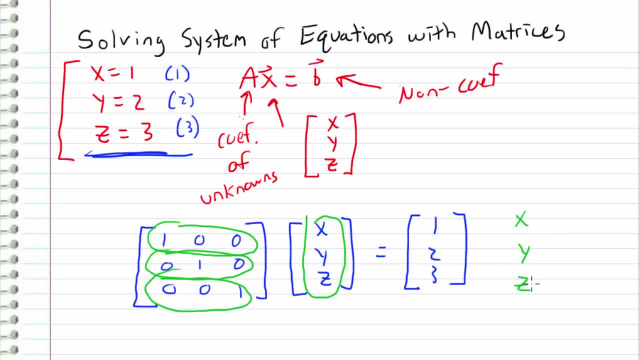 I were to take this third row, what I would get is Z, so the resulting vector from this matrix, multiplication with this vector, is XYZ, and this is equal to this vector: 1, 2 & 3. so we can see that we do have three equations We have: x is equal to 1,, y is equal to 2, and z is equal to 3,. 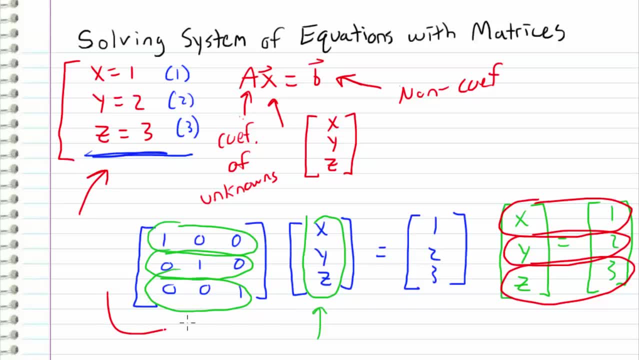 which is exactly what we started up here. So we know that this is, in fact, a valid representation of this system of equations, And the reason why I wanted to illustrate this is because I wanted to show you guys that we can represent systems of linear equations using the form ax is equal to b. So now let's. 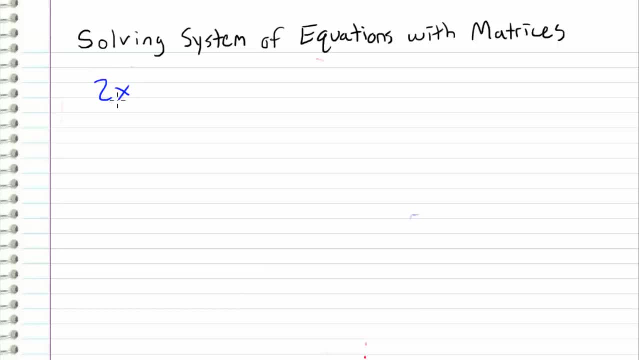 consider a less trivial example. Let's say that we have: 2x plus y plus z is equal to 1.. And then we have 4x plus 2y minus z is equal to 2.. And then, finally, we have 6x minus y plus 2z is equal to 4.. So we have 1,, 2, 3 equations And we have: 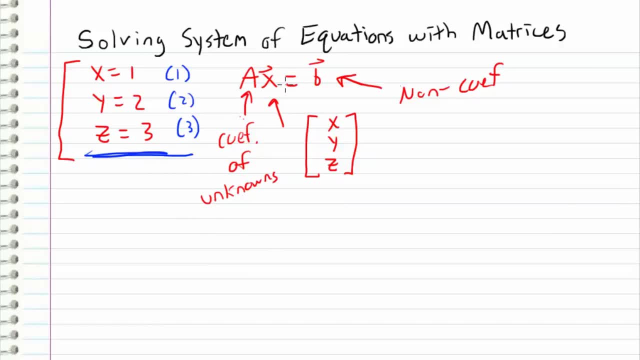 to organize this system into a, x is equal to b. well, I can do that like this Times: x, y, z, and this is going to equal the right hand side of our equation 1,, 2, and 3.. And let's verify that. 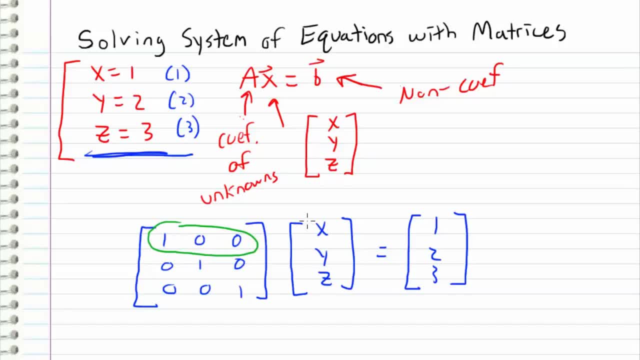 this is in fact true. If I were to take this first row and multiply it by our vector, what I would get is x. And if I were to take this second row and multiply it by our vector, what I would get is y. And then, if I were to take this third row, what I would get is z. So the resulting vector. 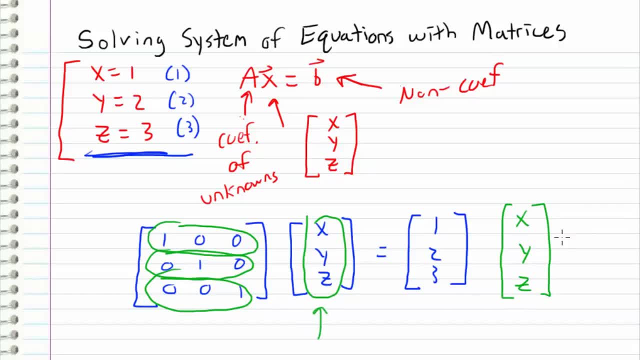 from this matrix. multiplication with this vector is x, y, z, And this is equal to this vector: 1,, 2, and 3.. So we can see that we do have three equations. We have x is equal to 1,, y is equal to 2, and z is equal to 3, which is exactly what we started up. 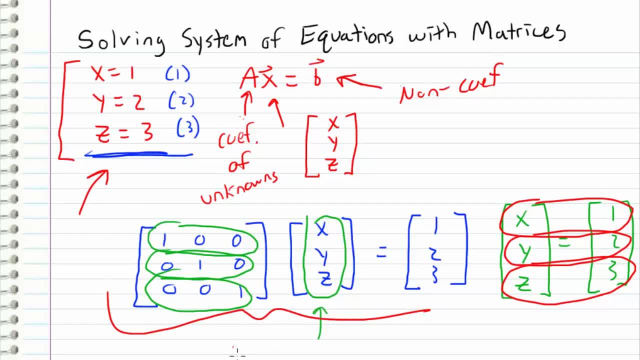 here. So we know that this is, in fact, a valid representation of this system of equations, And the reason why I wanted to illustrate this is because I wanted to show you guys, that we can represent systems of linear equations using the form ax is equal to 0. 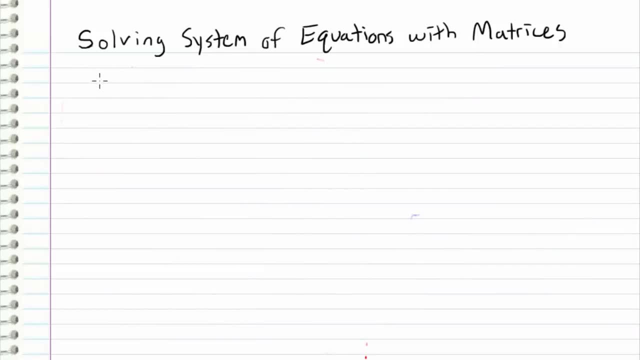 to b. so now let's consider a less trivial example. let's say that we have 2x plus y plus z is equal to 1, and then we have 4x plus 2y minus z is equal to 2, and then, finally, we have 6x minus y plus 2z. 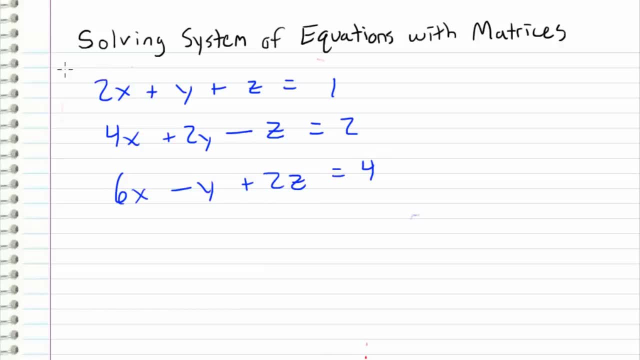 is equal to 4. so we have one, two, three equations and we have three unknowns, which are x, y and z, and now we want to solve for our unknowns x, y and z. so if you guys are coming from an algebra background then you may say: okay, we can do that by adding and subtracting multiples of our equations. 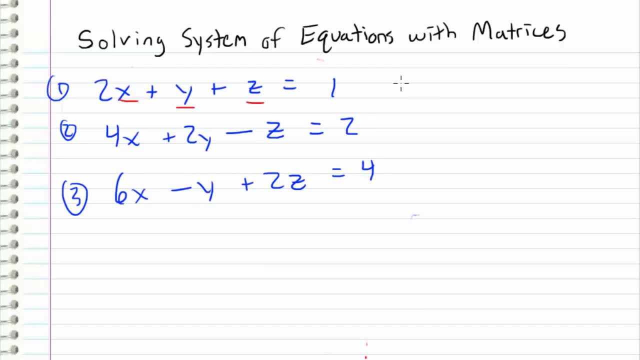 and substitution. like we can solve this first equation for x, y and z, and then we can do that by adding and subtracting multiples of our equations x in terms of y and z, and then we can plug that in here and then we can also do the same right. 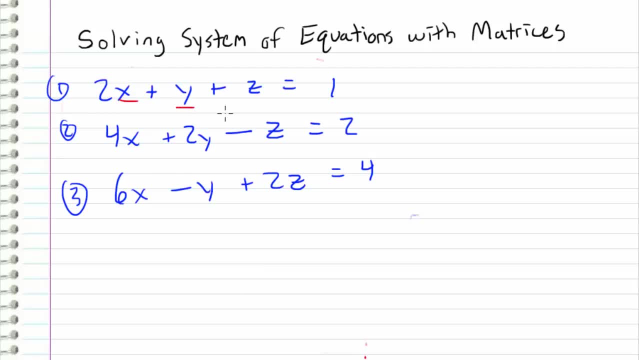 3 unknowns, which are x, y and z, and now we want to solve for our unknowns x, y and z. so if you guys are coming from an algebra background then you may say: okay, we can do that by adding and subtracting multiples of our equations and substitution. like we can solve this first equation for x in terms of y and 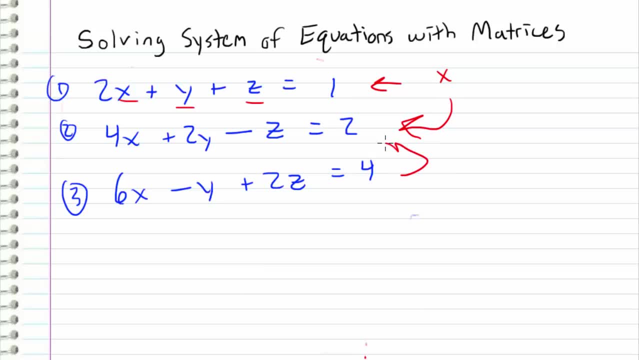 z and then we can plug that in here, and then we can also do the same right here and plug it in here and you get a mess. it takes a long time and it is tedious work and chances are you're going to make a mistake. instead, what we can do is we can solve this system using matrix equations, so I can. 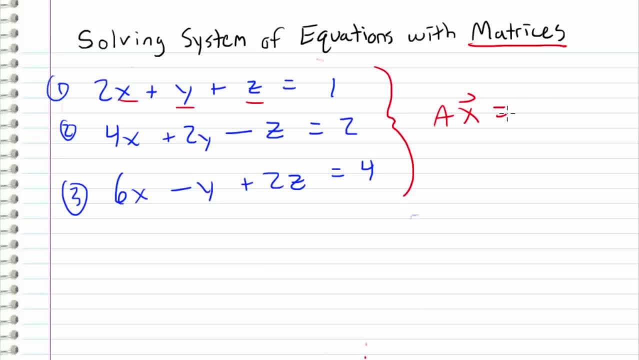 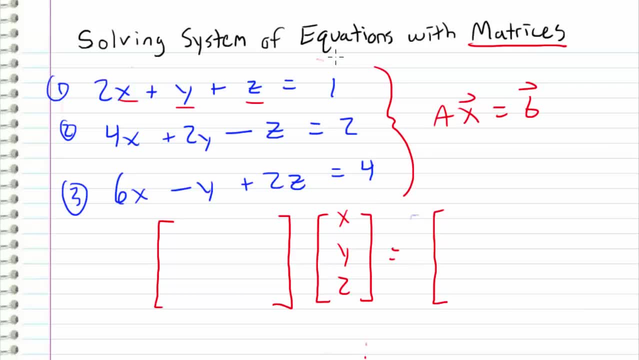 and this is going to equal the non-coefficient numbers which correspond to this right hand side, one, two and four. so now we just need to figure out where the numbers go and and make sure that the correct numbers are in the correct placement. so in this first equation we have 2x plus y plus. 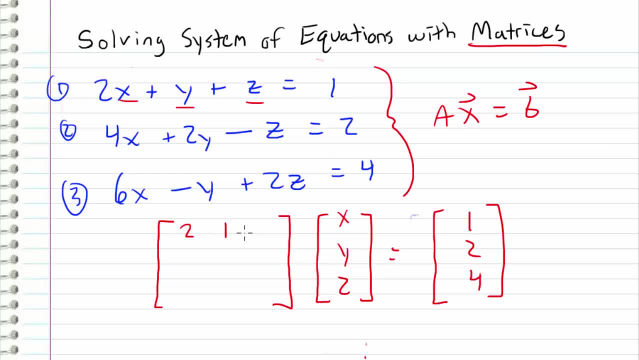 C is equal to 1. therefore I need a 2 right here, a 1 right here and a 1 right here, which correspond to two, one one. and then in the second row I have a four, a two and a negative one. so I put a 4, 2 and negative 1 right here, and then in the last equation I have a 6 negative 1 and a 2. so 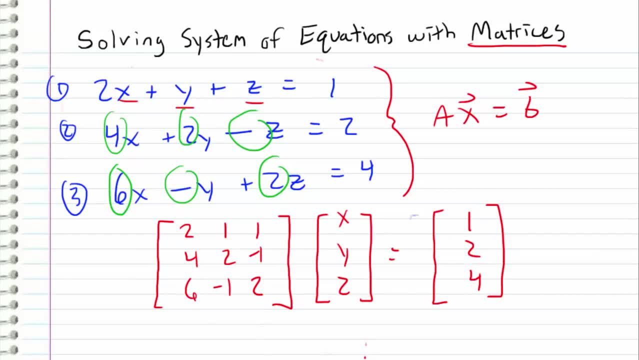 I put a 6 negative 1 and a 2 right here, and let's go ahead and verify that this does in fact represent our system. if I were to take this first row and multiply it by a vector, what I get is 2 times x plus 1 times y plus 1 times e, which comes out to be 2x plus y plus z. yep. 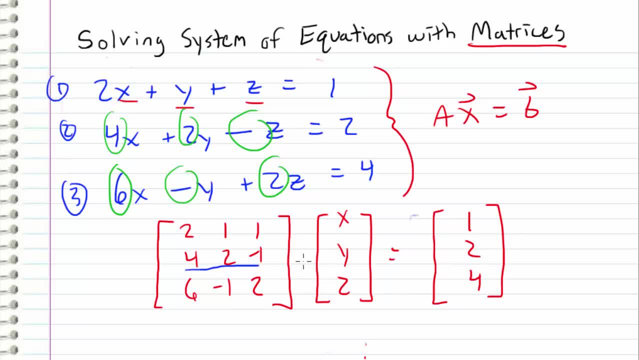 that's fine, and same thing right here. if I were to look at this row and multiply it by our vector, what I get is 4 times x plus 2 times y minus 1 times e, which is exactly what we get in our second equation up here, and we can verify the same thing for our last equation. so basically, 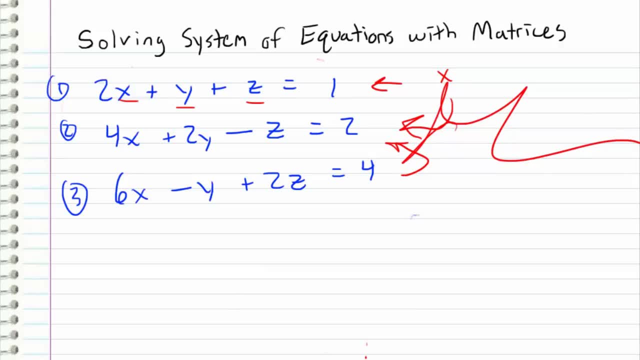 here and plug it in here and you get a mess. It takes a long time and it is tedious work and chances are you're going to make a mistake. Instead, what we can do is we can solve this system using matrix equations. So I can express this system in terms of: ax is equal to b, So the way that I do. 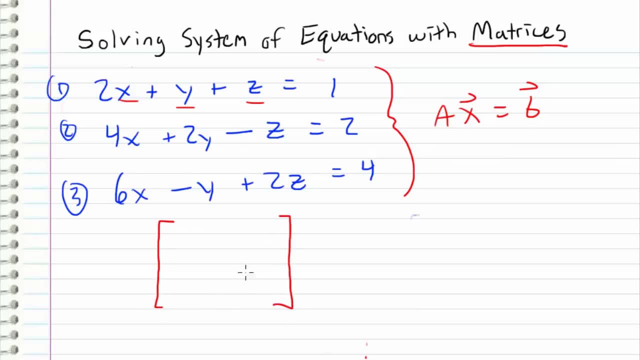 that, as I demonstrated before, is I put all the coefficients of our unknowns inside our matrix a and I multiply it by x, y and z, and this is going to equal the non-coefficient numbers which correspond to this right hand side: one, two and four. So now we just need to figure out where. 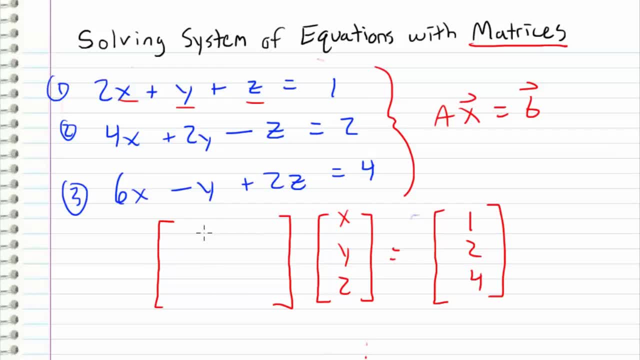 the numbers go and make sure that the correct numbers are in the correct placement. So in this first equation we have: 2x plus y plus z is equal to 1.. Therefore I need a 2 right here, a 1 right here and a 1 right here, which correspond to 2, 1, 1, and then in the second, 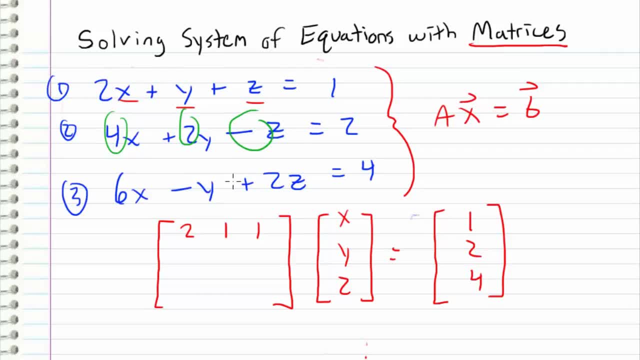 row, I have a 4, a 2 and a negative 1.. So I put a 4- 2 and negative 1 right here. and then in the last equation, I have a 6 negative 1 and a 2.. So I put a 6 negative 1 and a 2 right here and let's go. 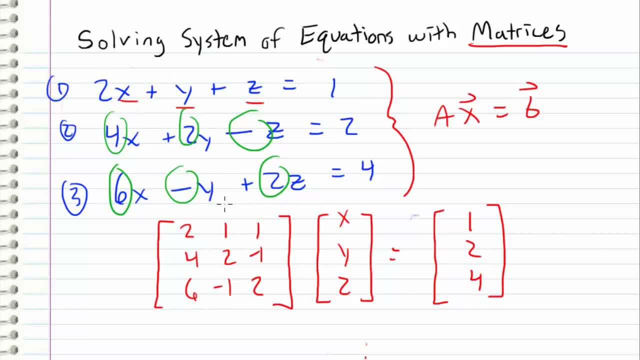 ahead and verify that this does in fact represent our system. If I were to take this first row and multiply it by a vector, what I get is 2 times x plus 1 times y plus 1 times z, which comes out to be 2x plus y plus z. Yep, that's fine and same thing right here, if I were to look. 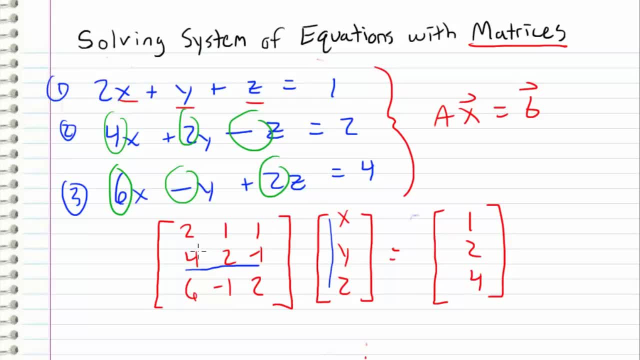 at this row and multiply it by our vector. what I get is 4 times x plus 2 times y minus 1 times z, which is exactly what we get in our second equation up here, and we can verify the same thing for our last equation. 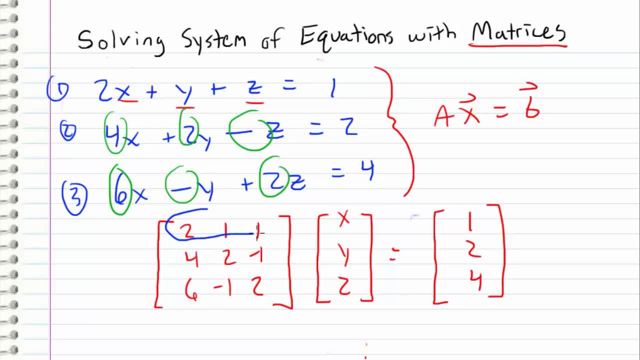 So basically, what we're going to do is we're going to take this first row and multiply it by a vector. so what we can see is that each row in this matrix system directly corresponds to the coefficients. up here in our actual equation, We have 2, 1, 1 and 1, and up here we have 2: 1, 1 and 1.